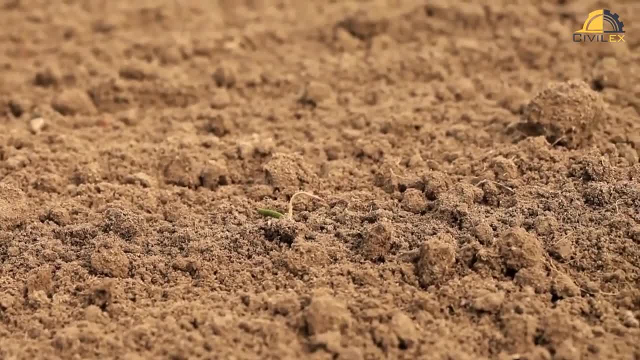 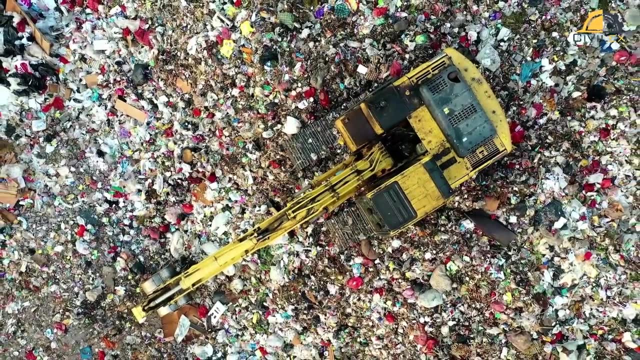 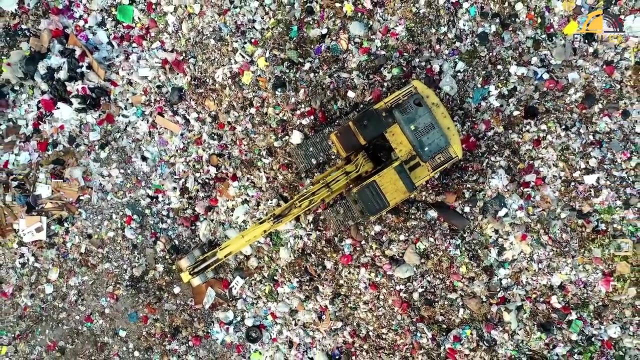 to cleanse the earth and make contaminated soil safe again. Let's get started. Our first technique is excavation and removal. When contamination is severe, this method involves digging up and removing the contaminated soil entirely. It's like hitting the reset button on a piece of land. 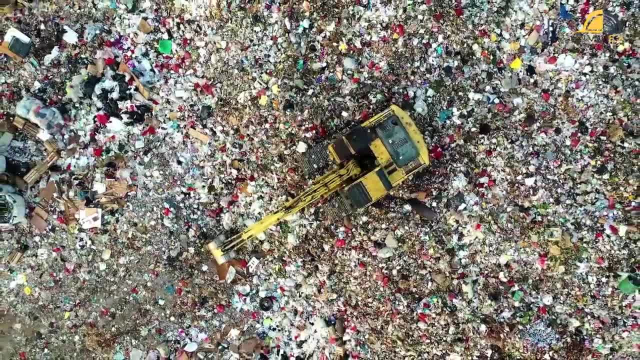 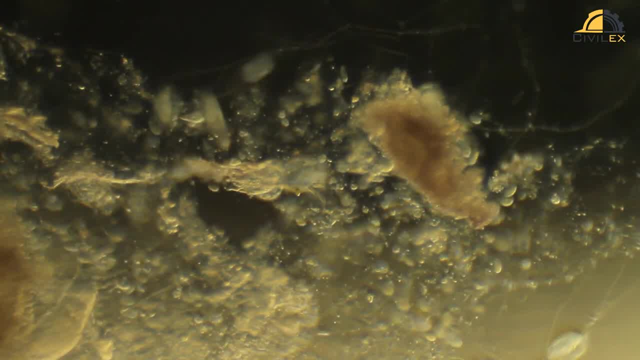 But remember, it can be costly and time-consuming. Now let's talk about bioremediation. Microorganisms like bacteria and fungi can be our earth's best friends. They break down and degrade contaminants, especially organic pollutants, making this method highly effective. Think of it as nature's cleanup crew. 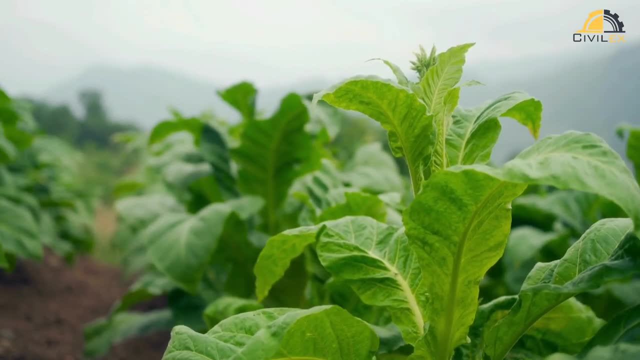 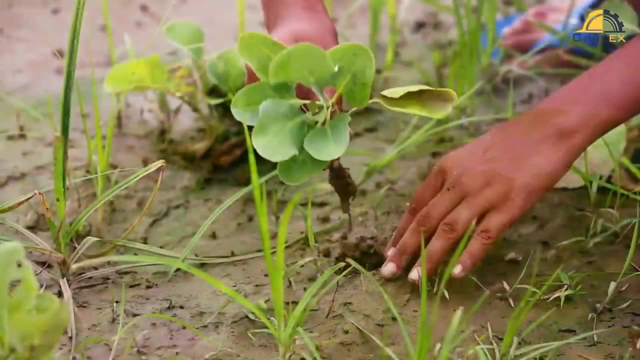 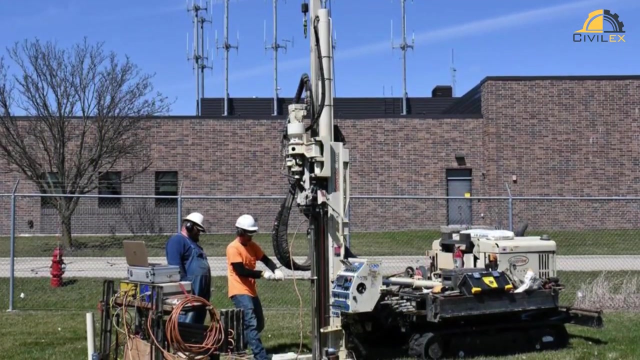 Moving on to phytoremediation, Certain plants known as hyperaccumulators have the superpower to absorb and store heavy metals in their tissues. Planting these superheroes can help cleanse soil contaminated with heavy metals. Chemical oxidation is another technique By injecting oxidizing agents into the soil. 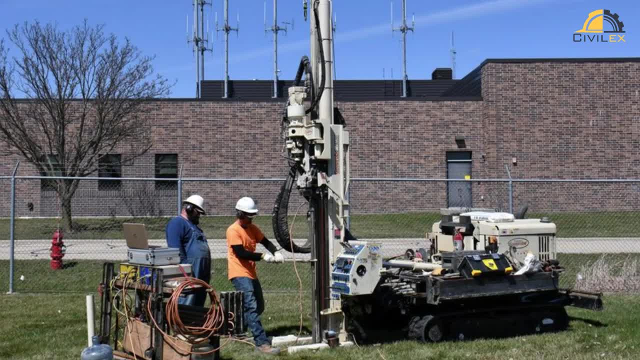 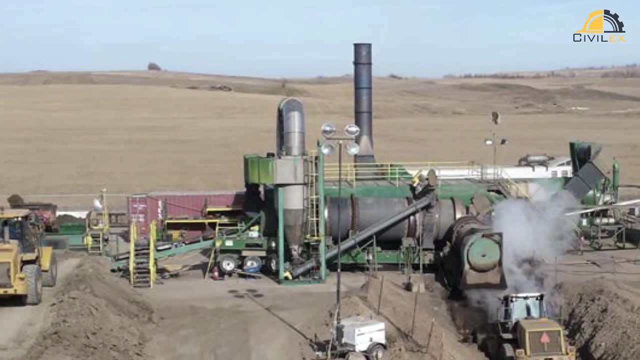 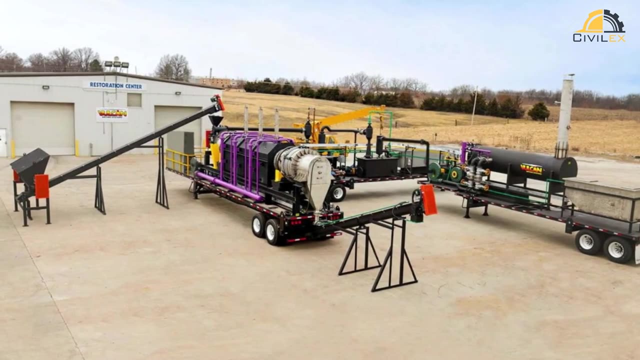 organic contaminants are broken down into less harmful compounds. It's like a chemical makeover for the soil. Thermal desorption is like sending the soil to a spa. We heat it to vaporize or separate contaminants, leaving the soil clean and refreshed. Soil washing uses water or cleaning. 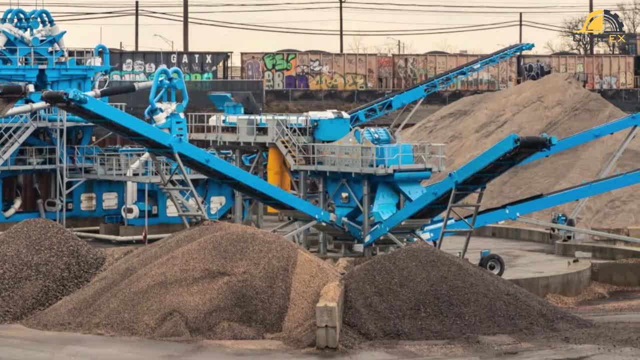 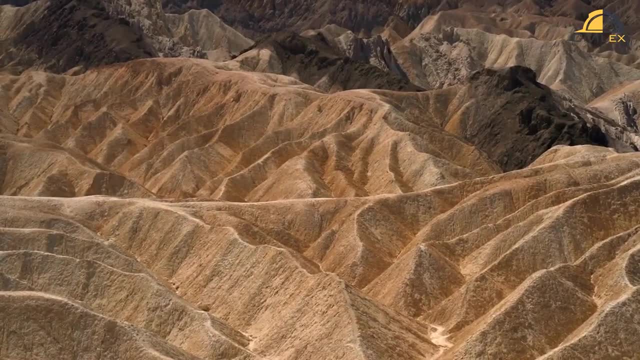 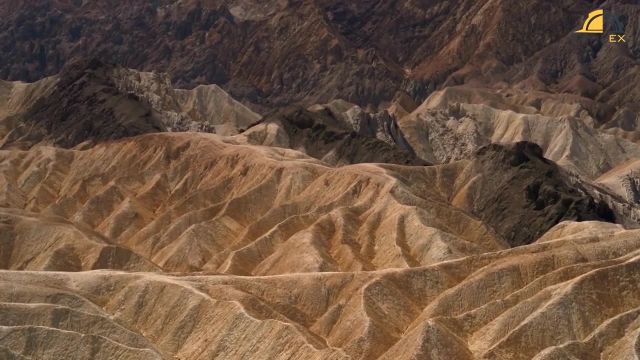 solutions to rinse away contaminants from the soil. The soil gets a thorough scrub and the wash water is carefully treated and reused. For sites where excavation isn't an option, in-situ remediation comes to the rescue, Techniques like in-situ bioremediation and 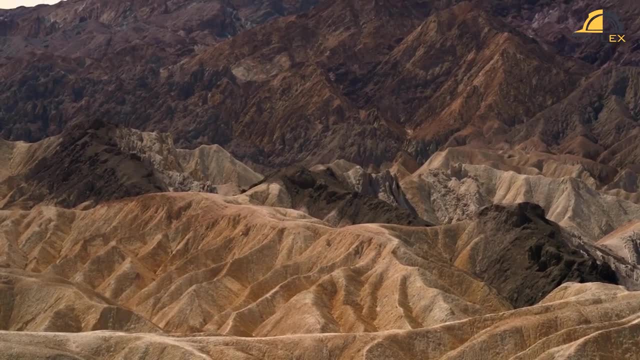 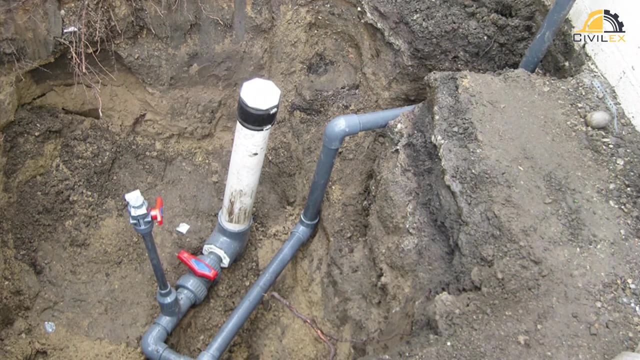 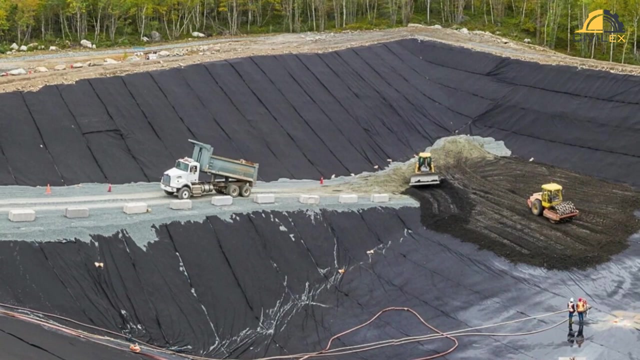 in-situ chemical oxidation treat the soil right where it stands. Vapor extraction is perfect for dealing with volatile organic compounds. We create a vacuum to pull out contaminants in vapor form for treatment. Solidification and stabilization are like giving the soil a concrete suit. 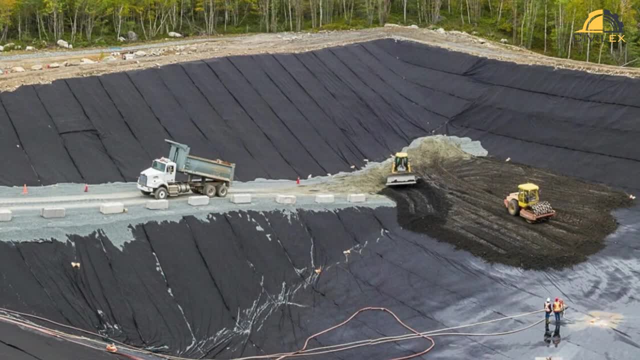 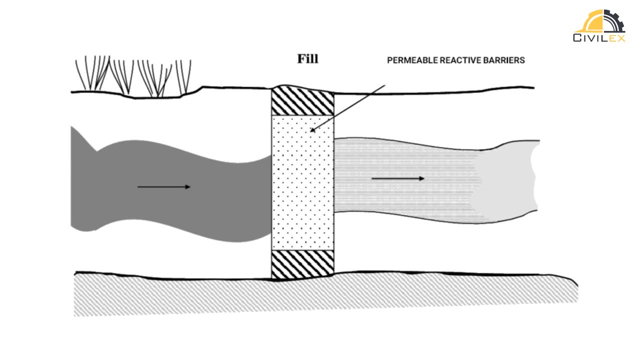 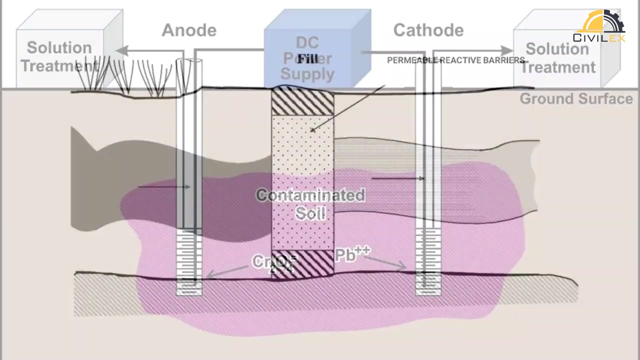 We add materials to immobilize or encapsulate the contaminants, making them less harmful. Permeable reactive barriers are our underground guardians. They intercept contaminants in their tracks, using materials like activated carbon to cleanse the earth. Last but not least, electrokinetic remediation uses electric currents to move contaminants towards collection points.